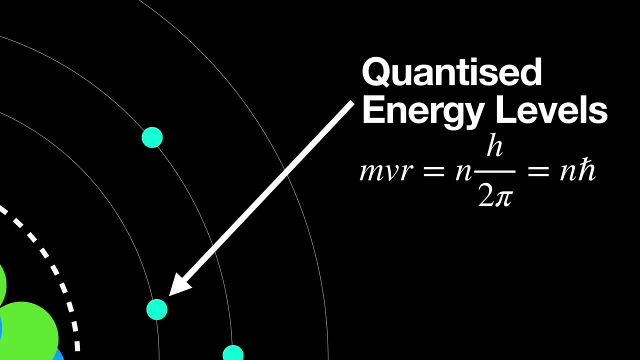 the angular momentum of the electron has to be some integer multiple of Planck's constant over 2 pi, commonly written as h-bar. He then used that assumption, along with some well-known classical physics, to come up with the radius of the hydrogen atom. That turned out to be correct In this video. 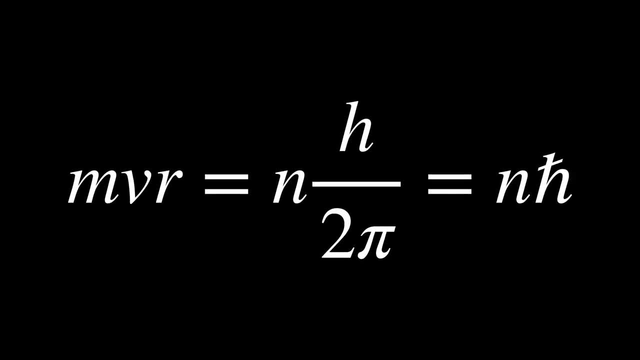 I'm going to try to do one better than Bohr and actually derive this postulate that he made. But first the basics. So imagine we have some electron around a proton and it's in circular orbit, undergoing circular motion, So basically the hydrogen atom. That means there must be a centripetal force acting on the electron around the proton, So basically the hydrogen atom. That means there must be a centripetal force acting on the electron around the proton, So basically the hydrogen atom. That means there must be a centripetal force acting on the electron And 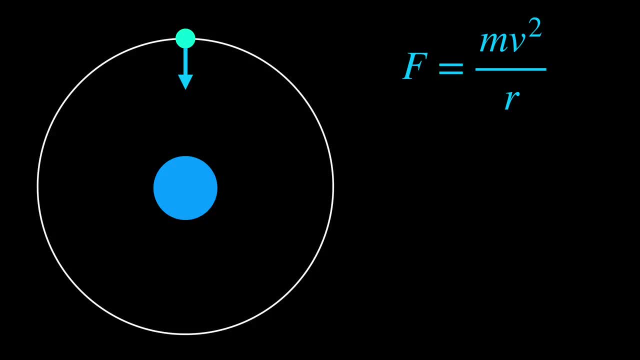 of course we know that the centripetal force is coming from the electrical force given by Coulomb's law, So we can just equate those. We can even plug in the values for the charges, since one is a positive elementary charge and the other is a negative elementary charge. 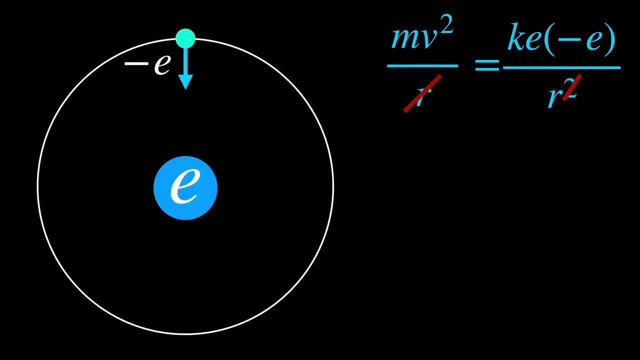 We can also go ahead and cancel some r's on both sides. Now we have the equation k times negative of the elementary charge squared over. r equals mv squared. I think it's fine if we just look at the magnitude of the force, so we can take the absolute value of both sides. 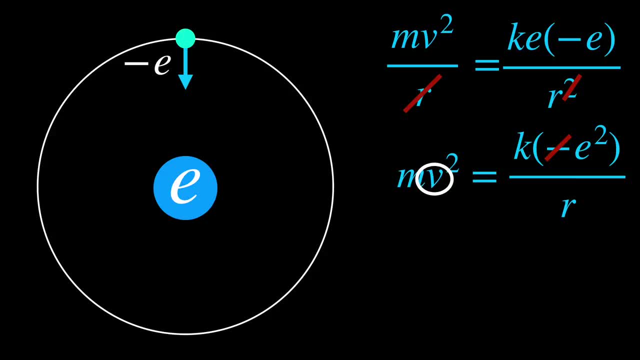 Now all we need is what the velocity of the electron is. So let's set this equation aside for a minute and come back to proving Bohr's postulate using the de Broglie wavelength, which I justify in another video which should be appearing above right now. 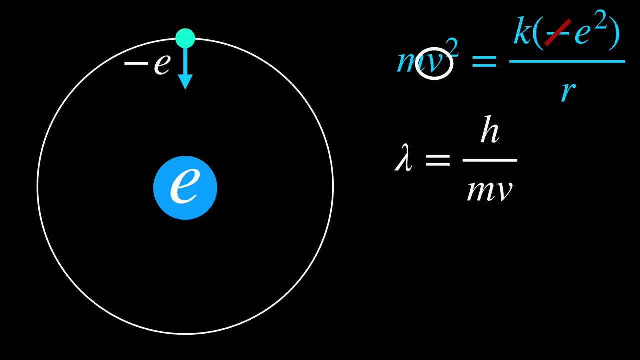 The idea that de Broglie pushed was matter waves, That is to say that particles are actually wave-like. If that were true, and it is then getting waves in an order orbit, seems like a weird idea, unless you use standing waves to just fit the waves around the. 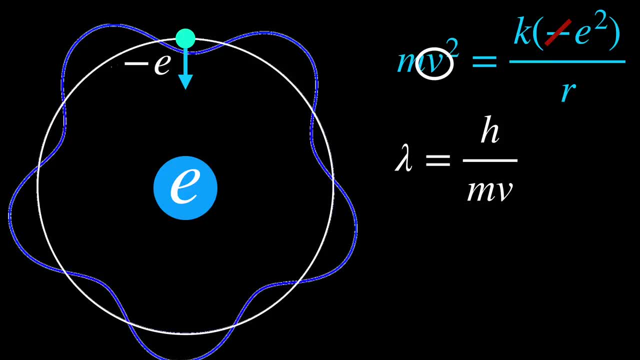 circle. In that case the circumference of the circle would have to be an integer multiple of the wavelength of the electron. Then we can just substitute in the expression for the de Broglie wavelength into lambda and rearrange for the angular momentum, mvr, by multiplying by mv on both.